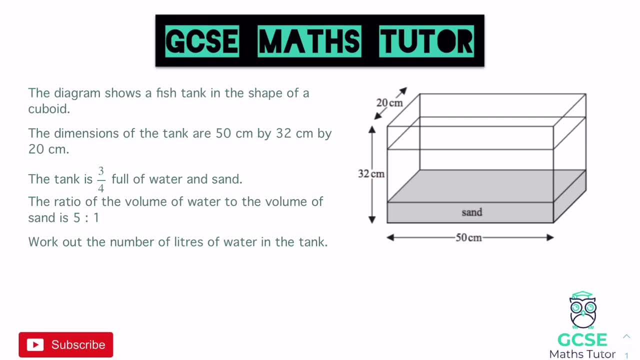 of discuss through them. As with all of these videos as well, please do like comment and subscribe if you haven't already. It really does help out with these videos and obviously you can comment and say if there are any other topics that you'd like to talk through or particular questions. 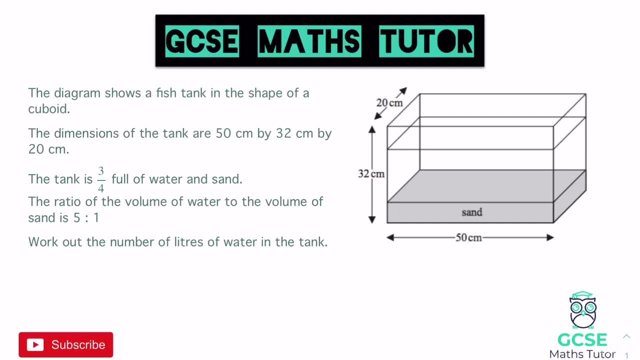 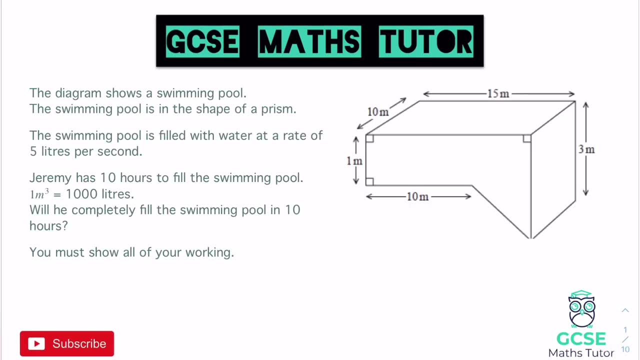 and I can always put them in place then for one of the next videos. But in regards to this video, I'm going to start with the first question. So it says here: the diagram shows a swimming pool and the swimming pool is in the shape of a prism. The swimming pool is filled with water at a rate of 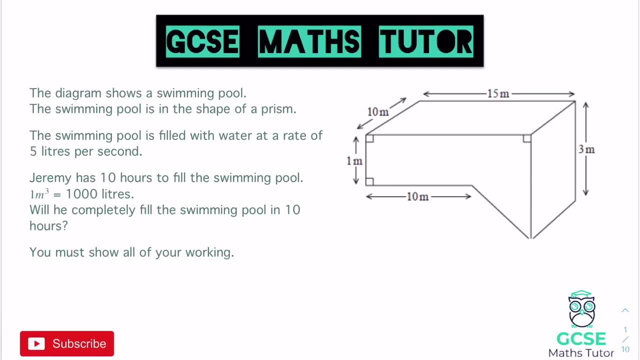 five litres per second. Then it says Jeremy has 10 hours to fill the swimming pool and one metre cubed is a thousand litres. Will he completely fill the swimming pool in 10 hours And he must show all you're working. There's quite a few different ways to approach this question, so 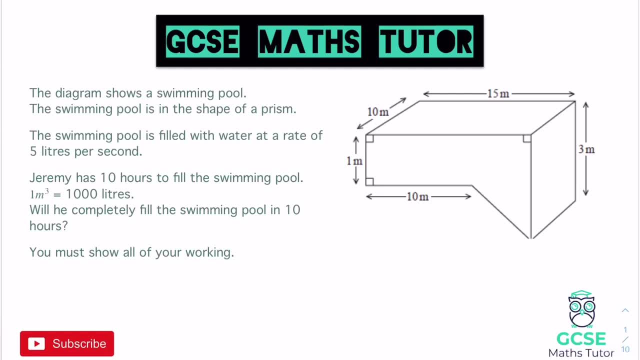 we'll have a little discussion about the different ways that you could approach it, but ultimately, with this type of question, what we really need to do is have a look at it and think: actually, what do we need to work out here? Now it's talking about the swimming pool being filled with water and it. 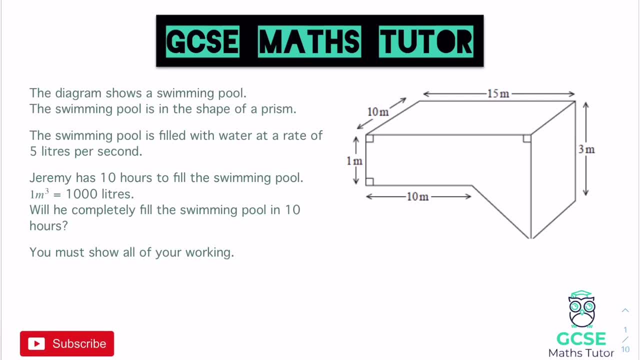 gives us lots of information about that and time and litres per second, and we've got some metric conversions there, but we're also going to need to just figure out what do we actually need to work out here? Now, if we're filling up a swimming pool with water, we're looking at the volume, okay, so 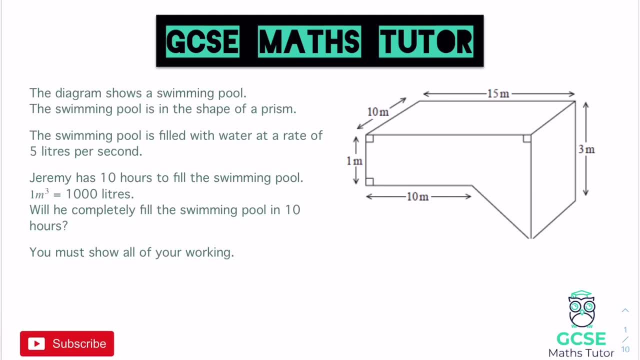 we're looking at how much water actually fits within this swimming pool, We're going to assume that it's filled right up to the top as well. So for having a look at this, then we've got a prism on the right and that's made up of two different sort of 3D shapes and, depending on which way we 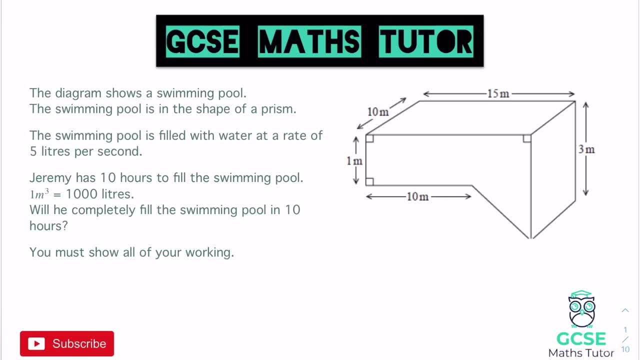 split it up. we could imagine that there's a big cuboid sitting on top, and if I draw on the diagram here, we could imagine there's a cuboid and on the bottom there's a triangular prism. Now, it's not the only way of splitting it up. we could split it up in lots of different ways I could actually get. 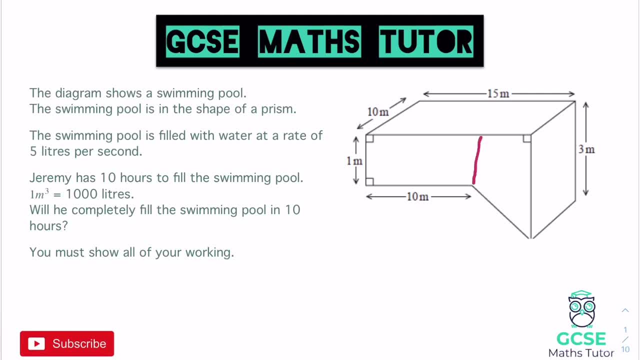 rid of that and I could split it this way and actually what we've got there is a cuboid on the left and a prism on the right that has a trapezium as its cross-sectional area there of the face on the front. okay, If we have a look at that, we've got a cuboid on the right and a trapezium on the. 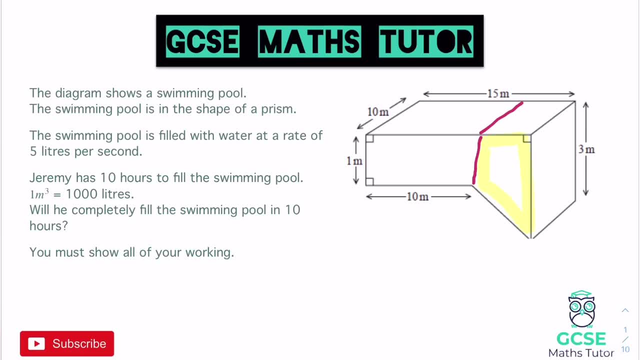 front. okay, If we have a look at that, we've got a cuboid on the left and a trapezium on the right. at this shape here that forms a trapezium. Now, I think just by the very nature of this question, 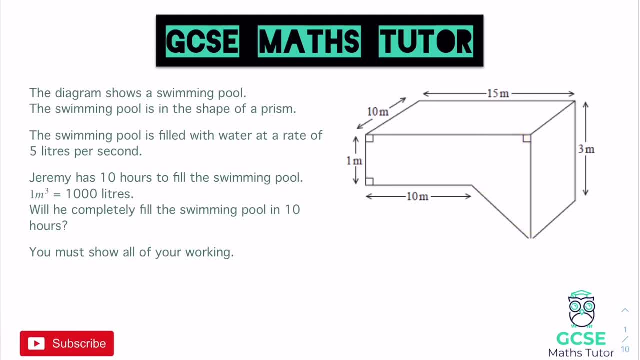 I think it's a little bit easier if we go for the cuboid and the triangle. I'd like to try and simplify it wherever we can, but we could do it in either way to work out the volume of the shape. So if I split it across and think about this as being a triangular prism and a cuboid, 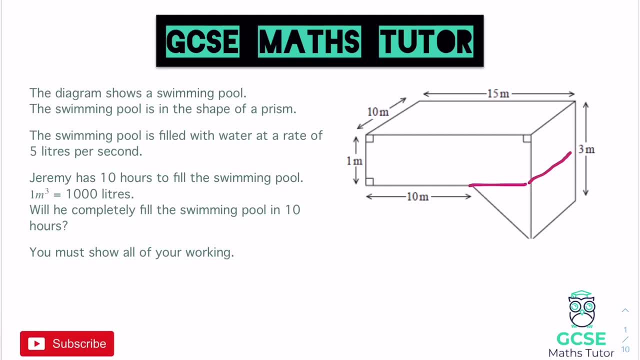 that's probably going to be our easiest approach. Now, once we've got the volume, we can have a look at tackling the rest of the question and breaking it down a little bit more. but in order to access any of this, we're going to have to work out its volume. 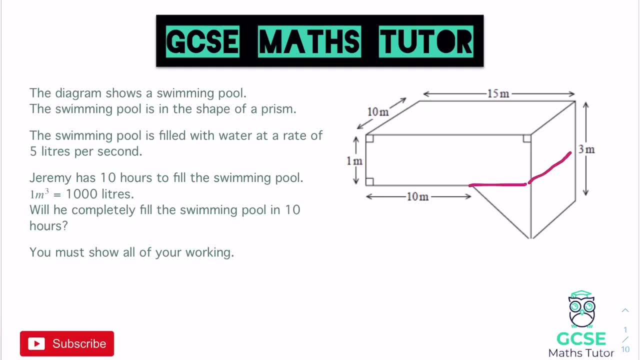 so we may as well start with that and forget about the other bits for the moment. Now looking at this, then, in order to work out the volume, we need to get the cross-sectional area. So by cross-sectional area- again, we're looking at this cuboid here. 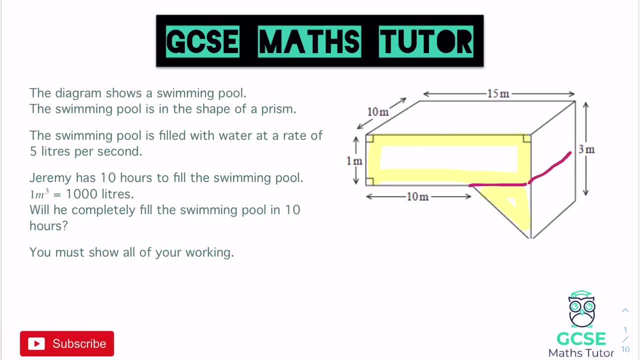 and then also the triangle that we have down there. So if we work these out separately, let's see what we get. So the cuboid's easy enough. I'm just going to write it on the front face. we've got a length of one going down the side and then a full length across the top. 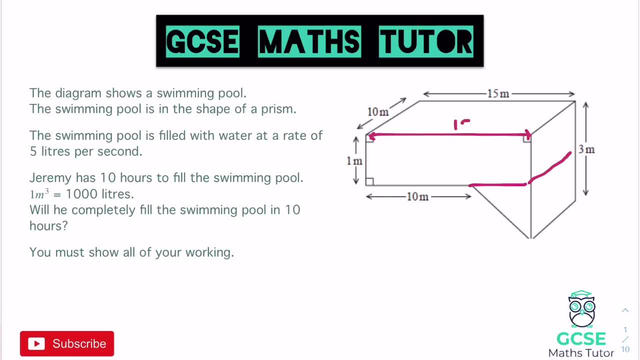 if we're looking at the full cuboid, 15.. So let's draw that in as well. So one times 15 will give us an area of that of 15.. We then need to have a look at the triangle. so the triangle- here we're going to have to find some of the lengths. for Now, if we have a look, 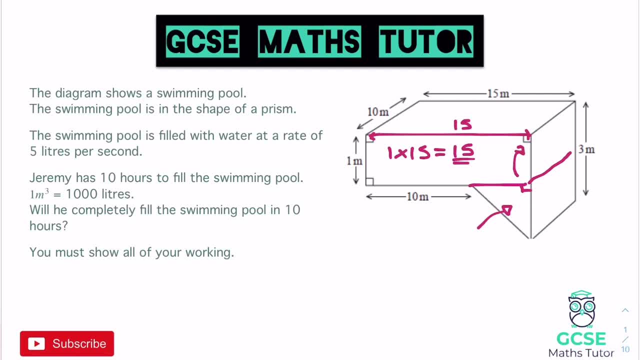 this here will be our right angle, as shown by the little right angle above there, So our base and height. we're going to want to have a look at these lengths here going down and then also this little length here going across. 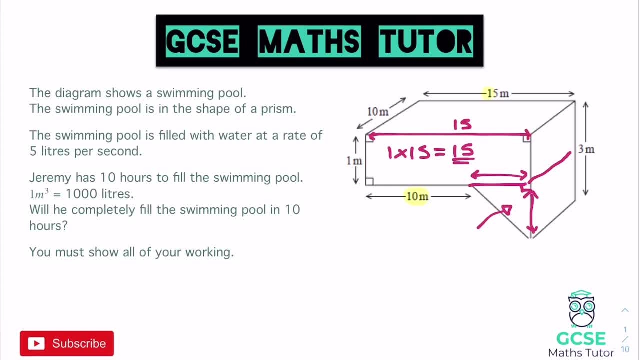 Now we know, obviously from the bottom here we've got a length of 10 and length of 15, so in order to actually access that length there, we're going to just have to find the difference between them. So that's going to be five meters here, and then the height there is. 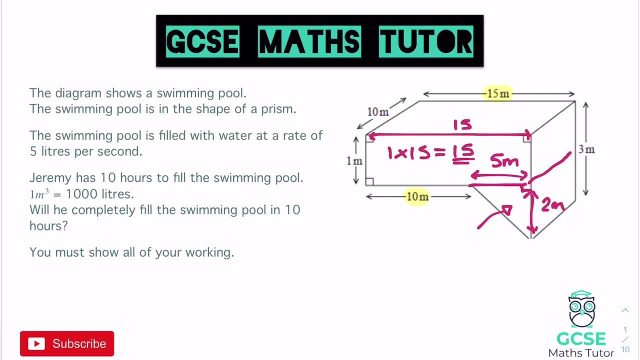 going to be a length of two meters So we can work out the area of that triangle. we know it's base times height divided by two or half base times height. but if we just do base times height divided by two we've got five times two, which is 10 divided by two gives us an area of five. 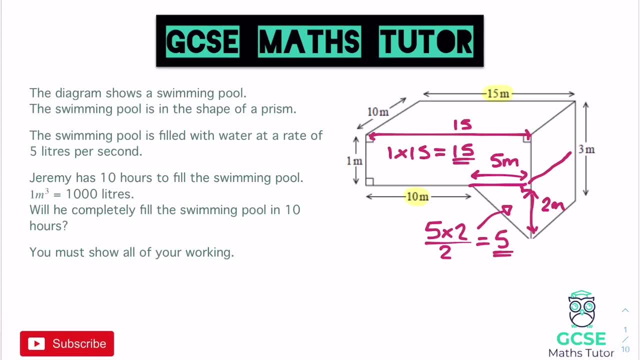 So there we go. we've got the area of the rectangle and the area of the triangle, So we have 15 and five and if we add those together we're going to get a cross-sectional area of 20.. So 20 is the area of the cross-section We know for working out volume. then and again, I'll link: 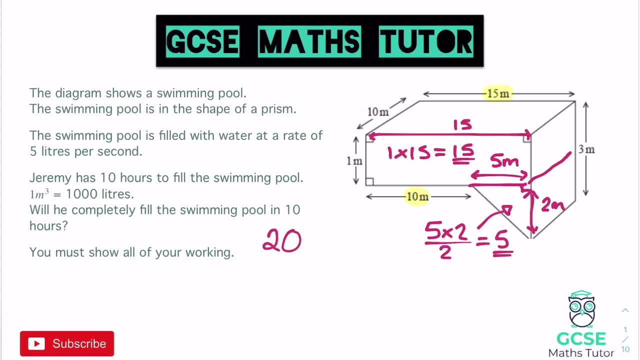 the videos for some of these in the description. we know to get the volume we multiply that by the depth, which in the case of a swimming pool is obviously the depth of the water. but in the case of a prism we're looking at the depth how far that cross-section. 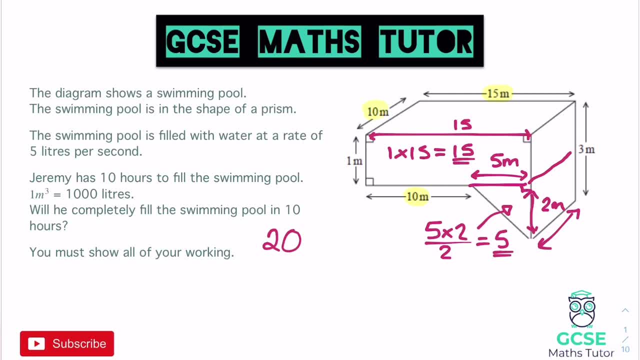 goes through the shape And that's given to us over here, on the left this time, which is 10 meters. So we're going to multiply that by 10, so 20 times 10 gives us our volume, which is 200 meters cubed. 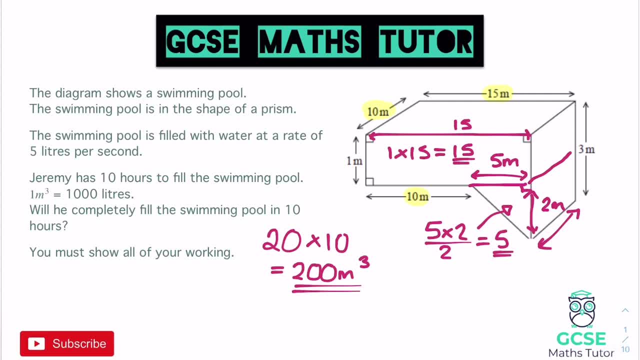 Okay, so there's our volume: 200 meter cubed. Now let's have a look at the rest of the question. So we've got some more information. it says the swimming pool is filled at a rate of five liters per second, and already that stands out because our units are in meter cubed. So that's going to. 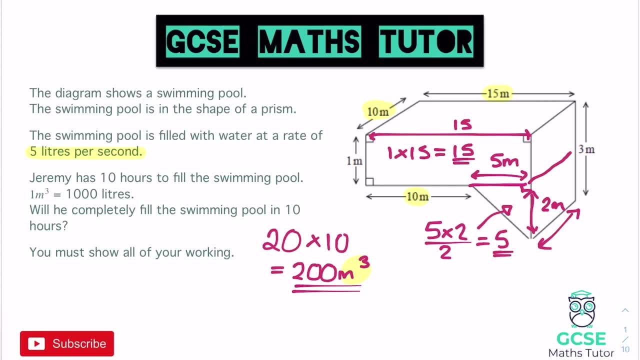 be something we're going to have to approach. It also says: Jeremy has 10 hours to fill the swimming pool. Will he compete? Correct? So we're going to completely fill it in 10 hours and we'll figure that out in a sec. 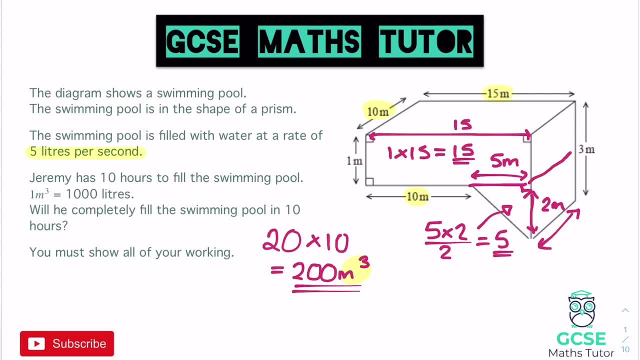 Now we've been given the metric conversion here, which is that one meter cubed is equal to a thousand liters. So in order to turn our volume here into liters, so that we can actually figure out how long it's going to take to fill the pool, we can change this meter cubed figure here into: 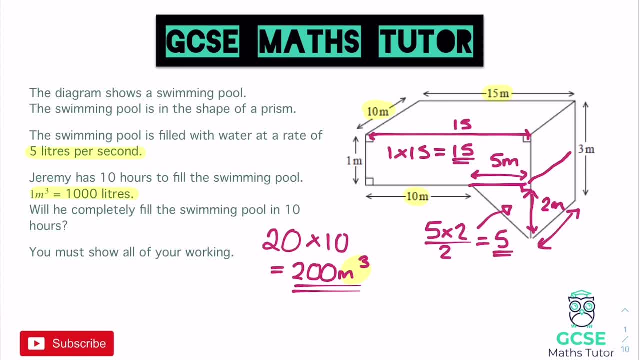 liters. So every one meter cubed is a thousand liters. So in order to turn that into liters, we can just multiply it by a thousand. Okay, every one of them is a thousand liters and we have to get 200 of them. So times that by a thousand and that gives us 200, with three zeros there. 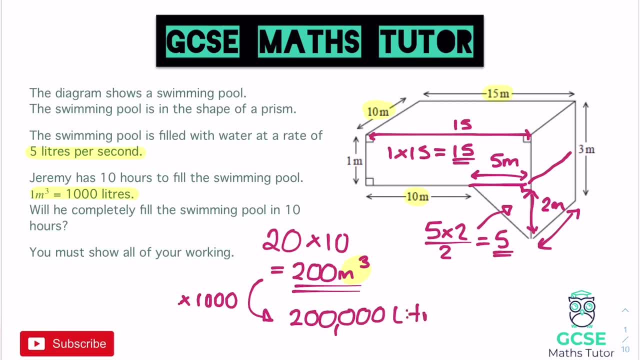 which is 200,000 liters. There we go. So there's our next step. We now have the pool in liters. We can now go about figuring out how long it's going to actually take to fill. So it says in the question there: it takes five liters per second And obviously we have 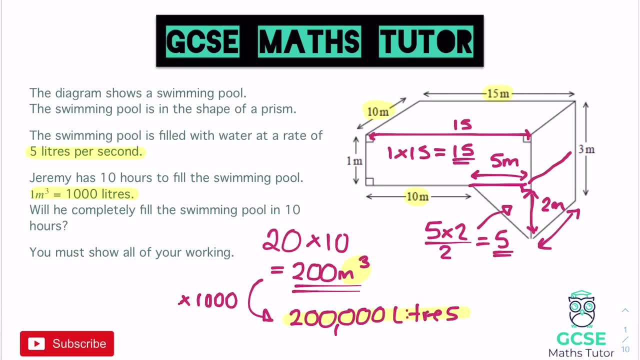 200,000 liters to fill up. So let's move this out of the way and let's figure out how we might get that now into an amount of time. Let's put that over there. Okay, so we have 200,000 liters Every. 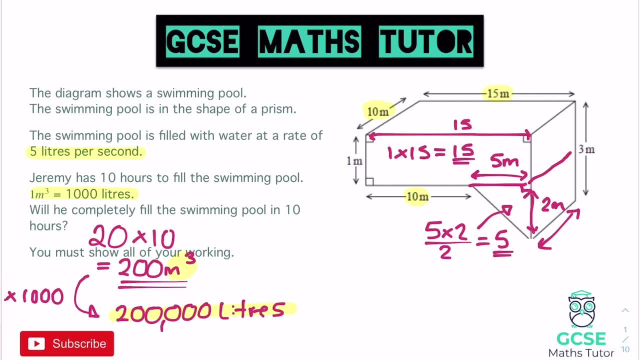 five liters is going to take one second. So in order to figure out how many seconds that's going to take, we're going to need to divide this number by five. So obviously, we're going to do this without a calculator for the moment, Although if you've got a calculator, that's fine to use. But 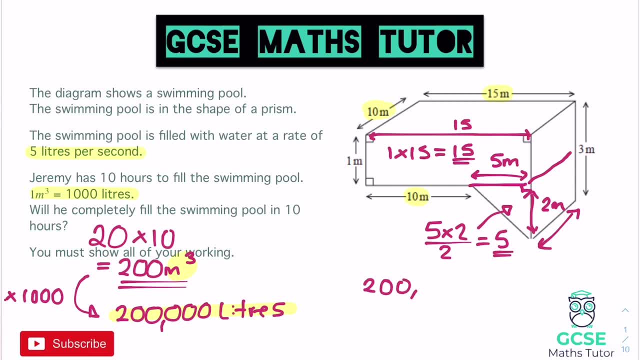 we're going to imagine this is a non-calculator question. So 200,000 and we'll divide it by five. There we go, And that's going to give us an amount of time. So that's going to give us an amount of. 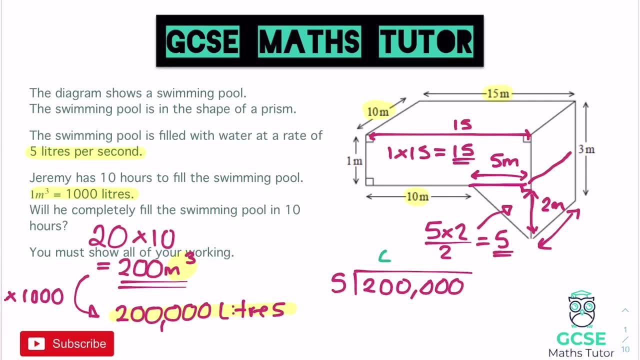 seconds. So five goes into 20 four times, And then we have the rest of the zeros, So 40,000.. So now we've got 40,000 seconds that the pool is going to take to fill. But it says here: 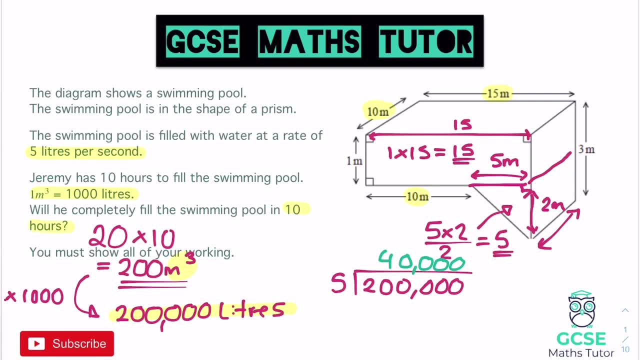 will it be full in 10 hours? So we know it's going to be 40,000 seconds And we want to compare that to 10 hours, So we need to figure out actually how many seconds there are in 10 hours or another. approach we could take. So we're going to take 10 hours and we're going to take the rest of the time. So we're going to take the rest of the time. So we're going to take the rest of the time. So we 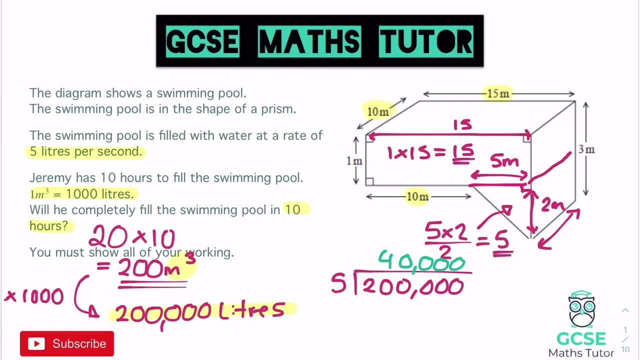 could turn 40,000 seconds into hours. We could start dividing it by 60 and turning it into minutes and then getting it back to hours. But I think the easier approach for this question is to actually turn the 10 hours into minutes. I think it's a lot easier here, particularly if 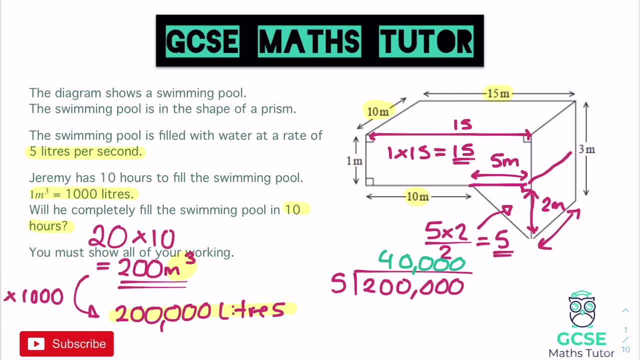 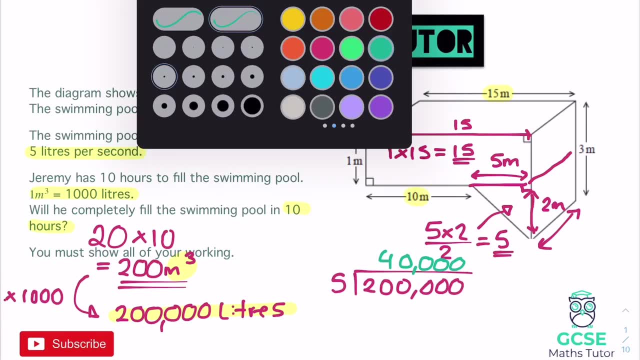 we're not using a calculator to multiply 10 and start turning that back into minutes than it is to start dividing 40,000 by 60. So let's have a look at this then. So if we've got 10 hours, we 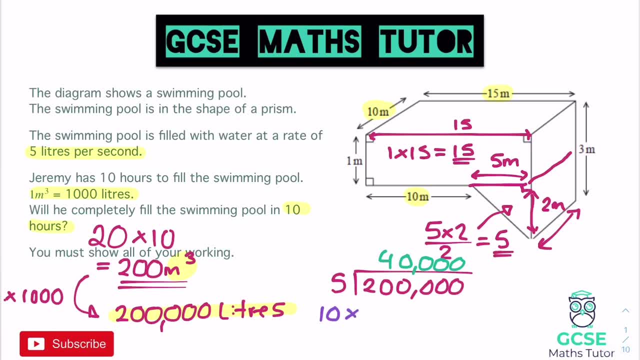 know there are 60 minutes in one hour. So if we times that by 60, that's going to give us the amount of minutes in 10 hours. So that's going to be 600 minutes, And then we want to turn that into. 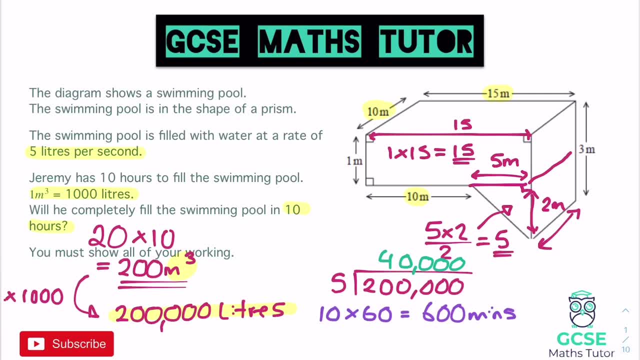 seconds to make a comparison, And we know there are 60 seconds in every minute. So if we do 600 and multiply that by 60, that's going to give us the amount of seconds in 10 hours. Now, six times six at the front is 36.. And then we have three zeros there, So that's 36,000. 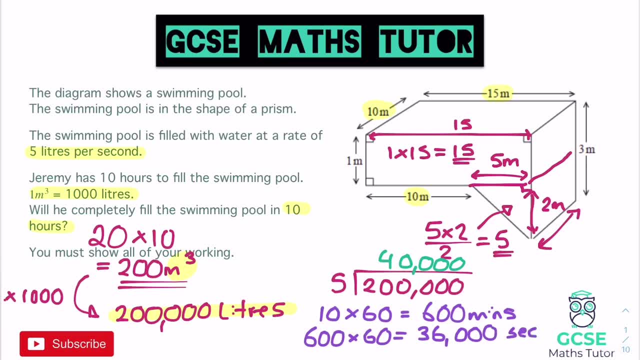 And that is seconds. So obviously, in the question here we worked out that the pool is going to take 40,000 seconds to fill and 10 hours is only 36,000 seconds. So, in terms of answering this question, look, the pool is actually going to take longer than 10 hours to fill, as it's 40,000. 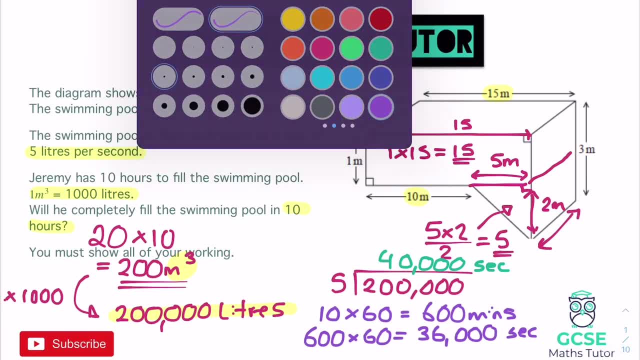 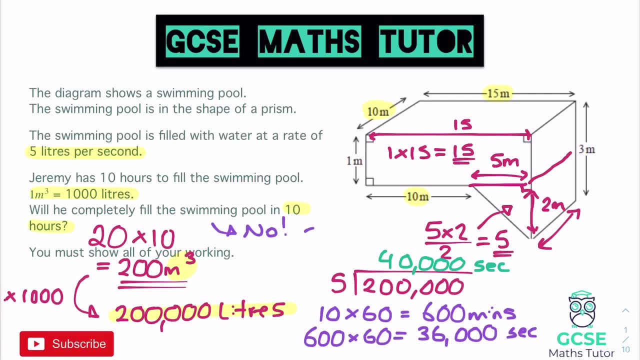 rather than 36,000.. So, in terms of finishing up our question here, we would say no, Okay, and then backed up by our question. So we would say no Okay, and then backed up by our working, because it's going to take 40,000 seconds and 10 hours is only 36,000 seconds. 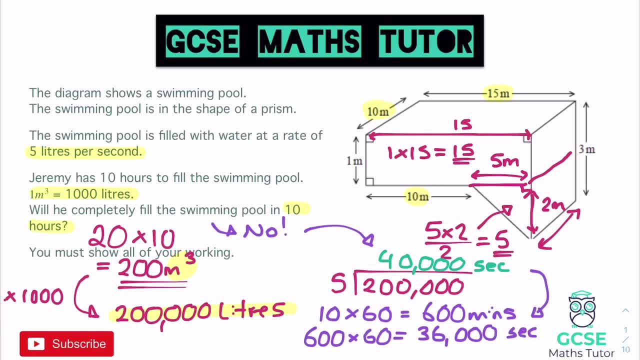 Now, obviously that's only one way of approaching it. As I said at the start, you could have actually split that question up into a trapezium and a cuboid instead. That would have been something different you could have done, And also in this question here you could have. 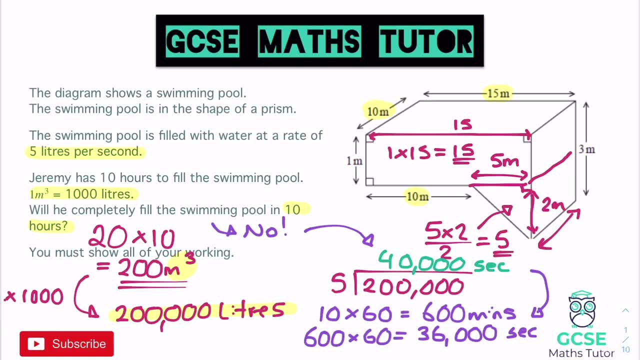 actually turned the 40,000 seconds into hours, obviously, which would have been a lot easier if you had a calculator, not so easy if you don't. But there was two different approaches there that you could have taken at different stages. But there we go. There's our first question. Now we're. 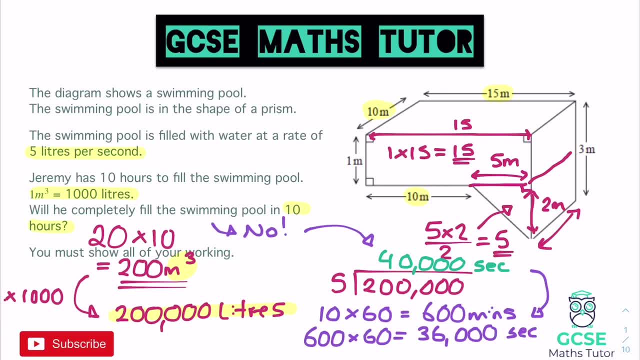 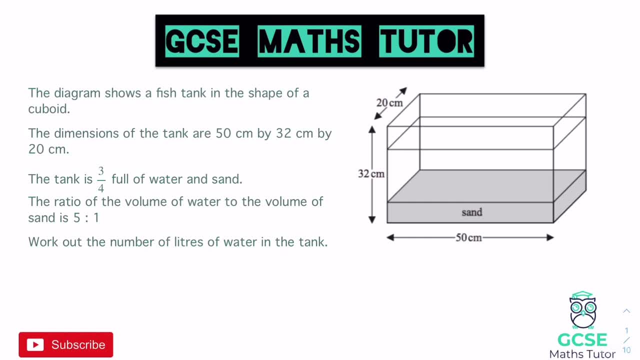 going to have a look at another question on volume, which is just a little bit different. Okay, so for this question we actually have an easier volume to work out, But the concept of the question is different again. It says here: the diagram shows a fish tank in the shape of a. 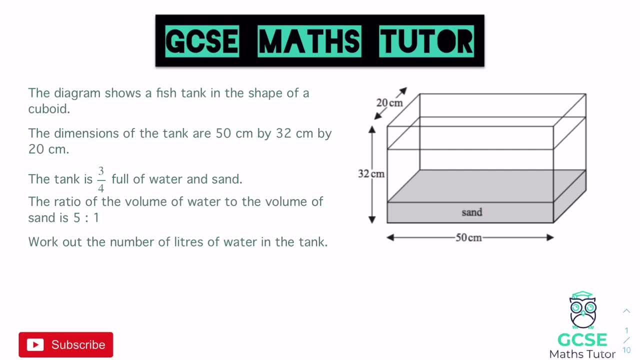 cuboid And hopefully we know with a cuboid the volume of that is obviously nice and easy for us to work out. It says the dimensions of the tank are 50 centimetres by 32 centimetres by 20 centimetres. 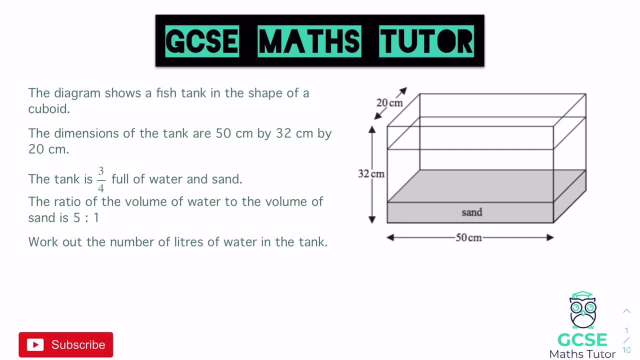 And again that's shown to us on the slide. So we've got a fish tank in the shape of a cuboid. It says the tank is three quarters full of water and sand, And again we can see that. And the ratio of the volume of water to the volume of sand is five to one. Work out the number of 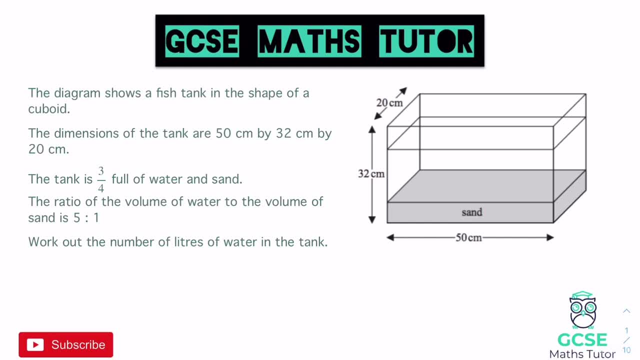 litres of water in the tank. Now, first thing first. what comes or stands out to me here is obviously that our units are given in centimetres and it's asking us about litres, So we're actually going to have to use one of our metric conversions here and actually figure that out for ourselves. 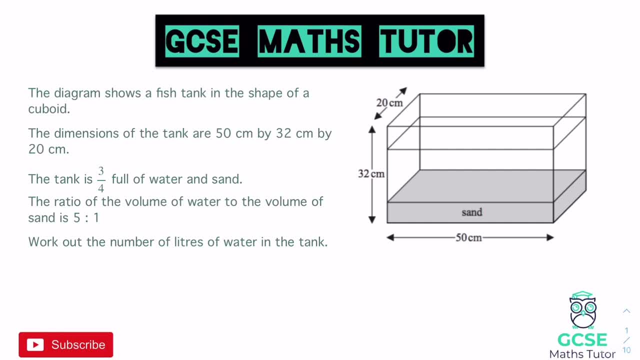 It's not been given to us. So it's something that we need to know in this question And we'll discuss that in a little bit. But for this question, here again we are looking at the volume of this tank And again there are two different ways that you could approach this. Now I think 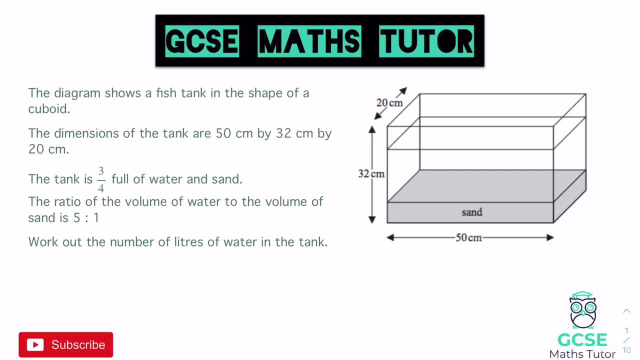 the easiest way to approach this is to first think about: well, what's the volume of the tank if it was full right to the top? And that's easy enough for us to work out, to get started on this question, And that's just to work out the volume of the cuboid. Now we know with working out volume, 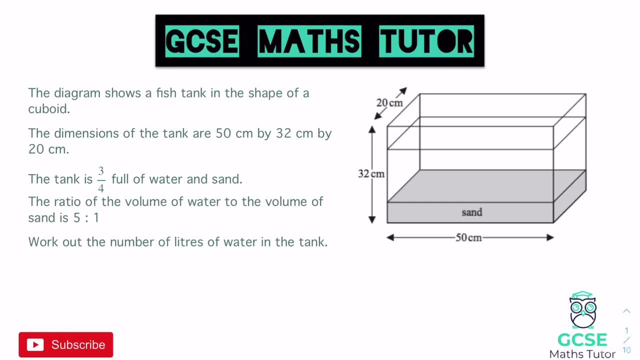 we need to work out the area of the cross section. When it comes to a cuboid, you can do a little cheat and you can just multiply all the numbers together. But we should really work out the area of the cross section and then multiply it by the depth. But in the case of this question, 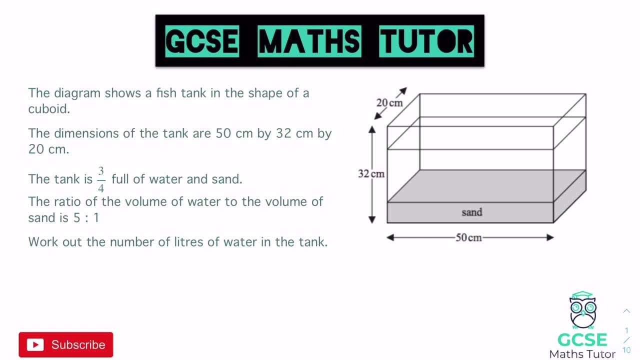 particularly as we're going to practice this non-calculator. I think it's actually easier- and I don't like doing it, but picking the two easier numbers to multiply, to start with 20 times 50. And if we do 20 times 50, 2 times 5 is 10.. Let's just write this down: 20 times 50.. 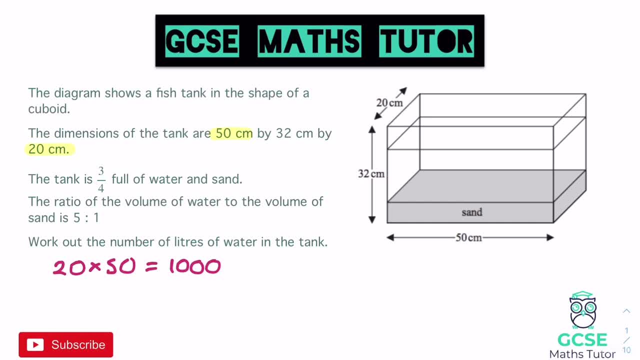 2 times 5 is 10. And add the two zeros And it comes to 1,000. And that just makes it nice and easy. to then multiply that by the 32. And to get the volume here we can do 32 multiplied by 1,000. And that gives us a total volume there. 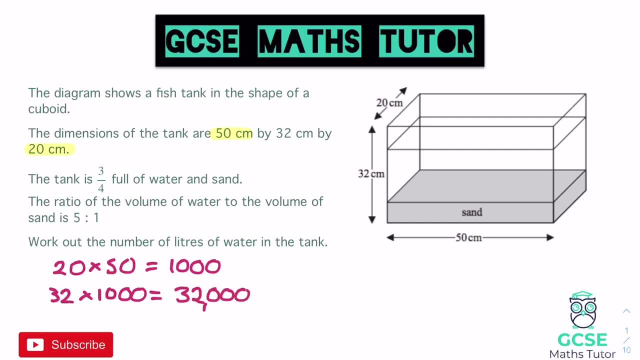 of 32,000.. There we go, And not forgetting our units there, that is a centimetre cubed. Now it's up to you what approach you take at this point. We could start working out, then, what three quarters of that is, to figure out what volume of the tank is actually filled up. 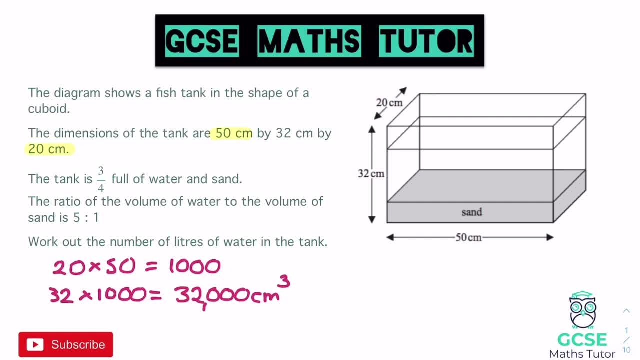 and then having a look at this ratio And, as you can see, obviously, although we've got volume involved, we've also got fractions and ratios and also conversions involved As well. as having to obviously break this all down Now, I think the easiest thing at this point. 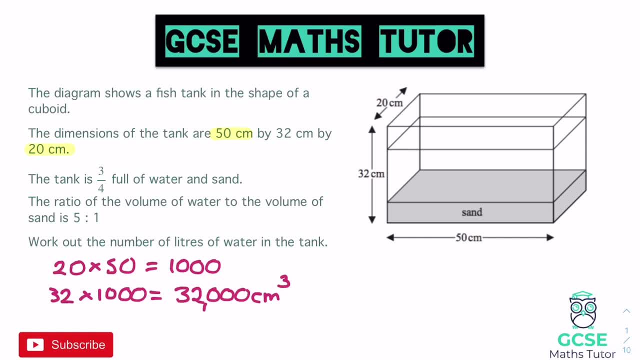 is probably just to turn this straight into litres, And the unit conversion that you need to know is 1,000 centimetre cubed, okay, is equal to 1 litre, Okay. so that's one of the important unit conversions that we need to know And it might not necessarily be given to you, So it is one. 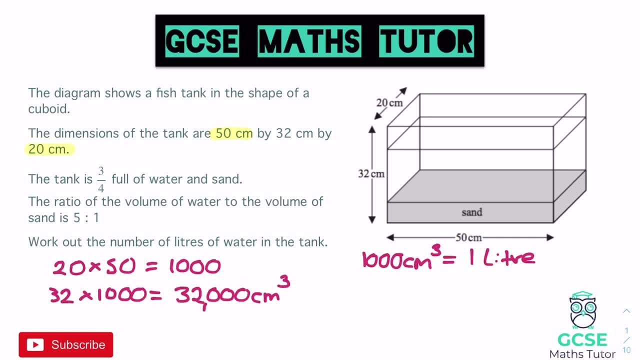 that you need to know, just like on the last one, that that 1 metre cubed was 1,000 litres. So for this one here, definitely a little key point to make sure that you've got there: 1,000 centimetre cubed is 1 litre. Now for the next stage of this. we need to obviously turn it. 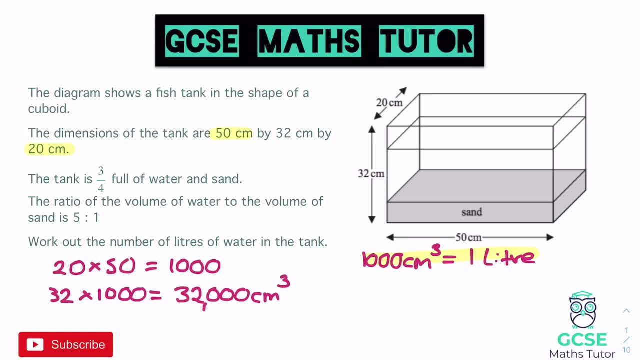 into litres. So in this sense we have 32,000 centimetre cubed. So if we want to turn that into litres- the opposite of what we did last time- this time we're going to divide it by 1,000.. 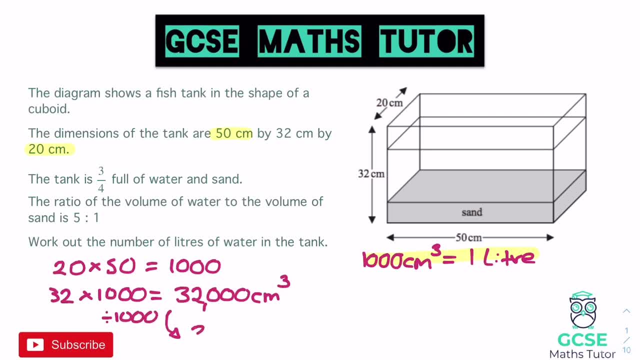 And if we divide that by 1,000, we can knock off the three zeros and we get 32 litres. There we go And there is the volume, The volume of our full tank. Now, obviously, the next piece of information in the question. 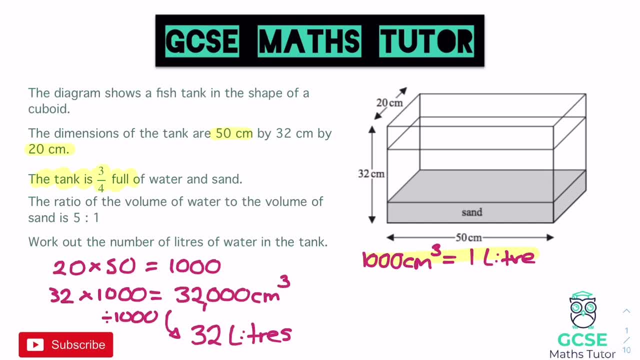 said to us that the tank is three quarters full of water and sand. So if we find three quarters of 32, we'll be able to find out what quantity there is actually the water and the sand. So if we find three quarters of 32, there we go, three quarters of 32.. And that's easy enough for. 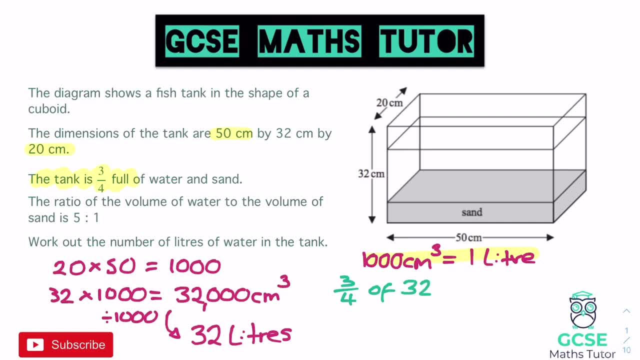 us to do? We just divide by four and times by three. Thirty-two divided by four is eight, Times that by three is 24.. So we have 24 litres. There we go. That's our water and sand. Now you can imagine at this point if I hadn't have done this conversion straight away. 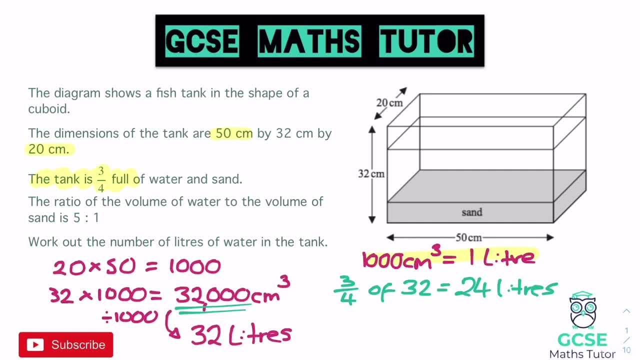 I would have had to have found three quarters of 32,000, which isn't necessarily more difficult, but it is a little bit more fiddly there with a larger number, So it's probably better for us to have made that conversion straight away. So just something to be thinking about in that question. 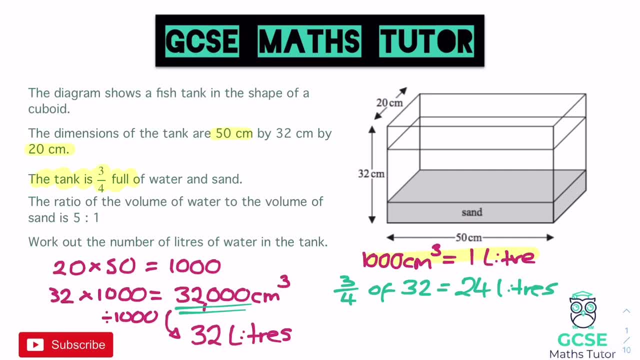 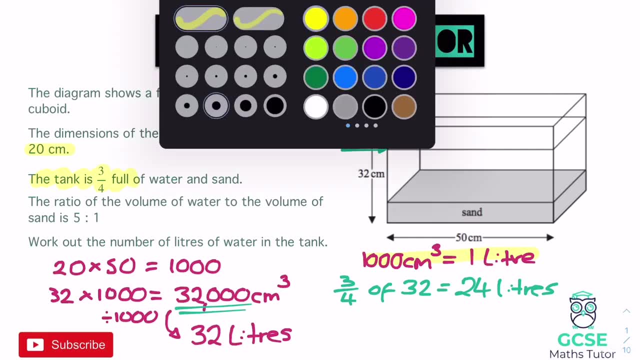 there We now know how much is full up with water and sand, So we can imagine that we have water and sand. OK, that's up to this point here where the water stops. And then it tells us in that last piece of information there that the ratio of the volume of water to the volume of 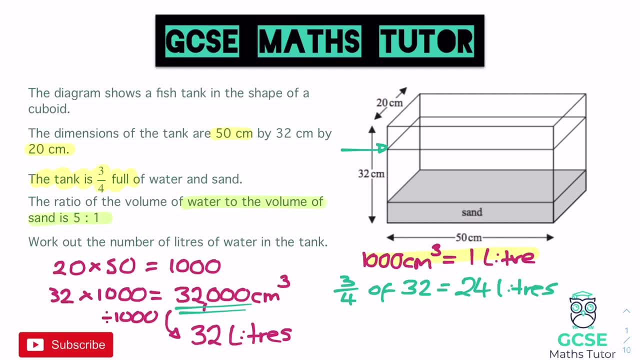 sand is five to one. So essentially all we need to do is take that 24 litres that we have and split it in the ratio five to one. Now, hopefully you remember. obviously, with ratios we're going to figure out how many parts there are in total, and that's six parts. So if we do 24 divided by six, 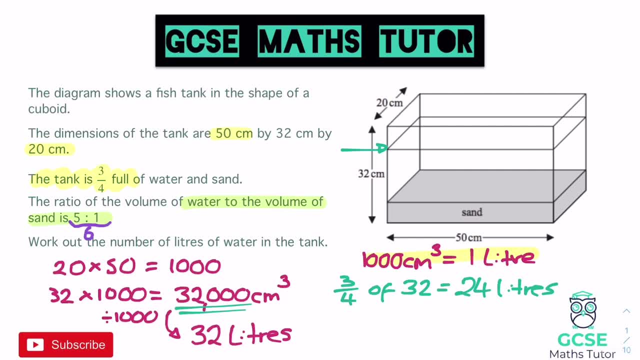 we'll be able to split that up in the ratio. Let's write this out. So five to one, I'm going to figure out what we're going. to multiply both of those by So 24 divided by six, our total amount of parts. there is four, So we're going. 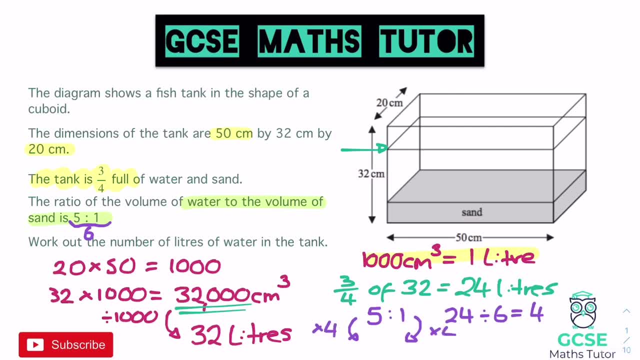 to multiply both of these numbers by four to get our corresponding litre values. So five times four is 20, and one times four is four. And again, remembering just a quick double check there- to add those two together, make sure it adds up to our original amount, which it does. 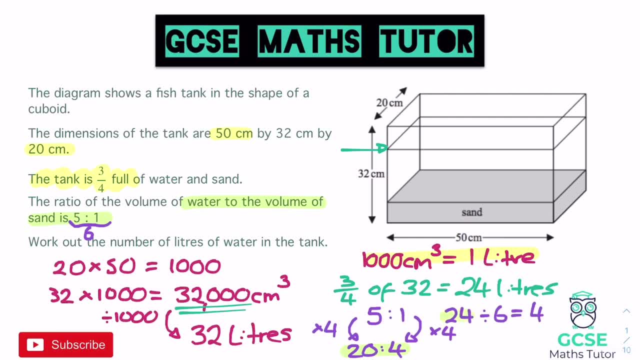 which is four. So, in terms of answering our question here, look, just remembering that the five was the water, the one was the sand, and it wants us to work out the number of litres of water in the tank, And we've got that right there: 20.. So there we go. Our final answer: there would be 20.